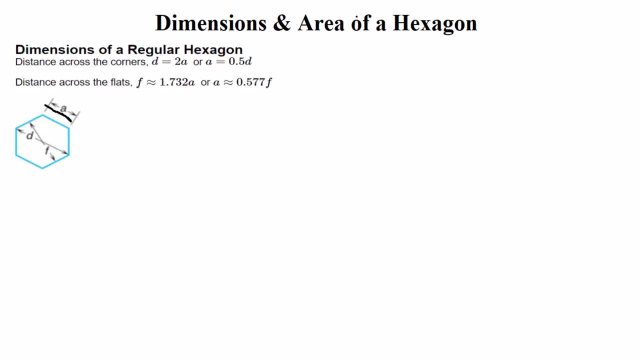 It's also important to know the different things about a hexagon, For example. so here I have a drawing of a regular hexagon, All right. so typically, if we're talking about a regular hexagon, a regular hexagon where all sides are equal, so one side is typically given. 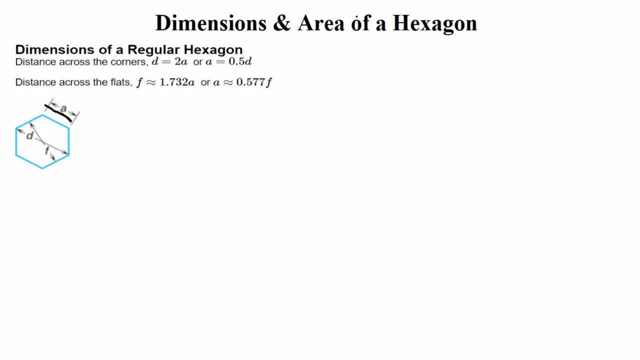 and that side is known as A right. So if you know what A is, you know all the other sides of the hexagon. so therefore you can find the perimeter of the whole thing right. Otherwise you might have to calculate the distance across the hexagon. 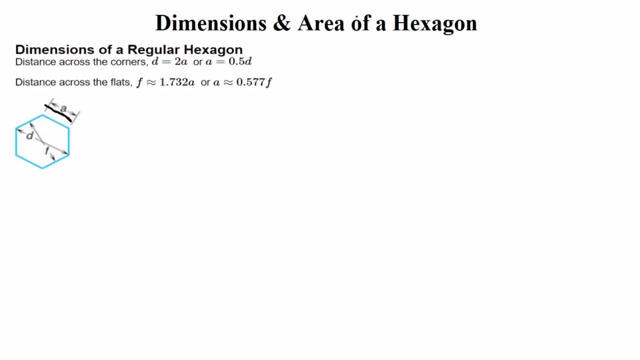 and there's two different ones that you can talk about. There's the distance across the corners right, And that is take a corner, a vertices here, all the way across to a vertices on the other side. So, corner to corner, that's called the distance across the corners. 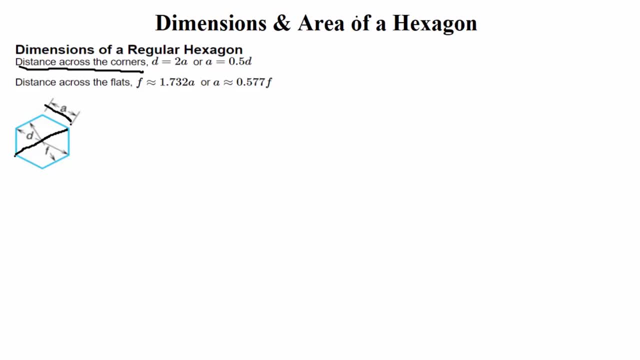 And in order to find the distance across the corner, we have these little formulas here: D is equal to 2A, So as long as you know what A is, the side of the hexagon, just multiply that by two and you're going to have the distance across the corners. 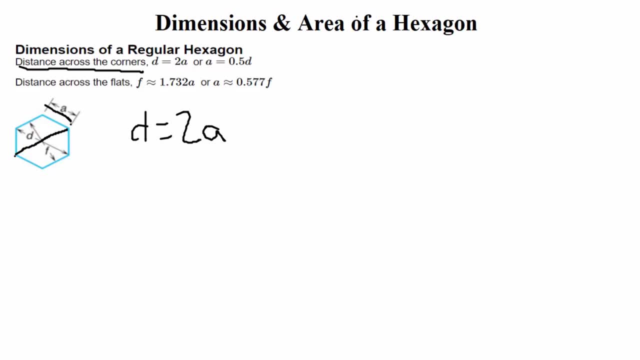 There's also distance across the flats and that's from the flat side of the hexagon across to the other flat side of the hexagon. So it's a slightly different calculation. So if you're going from the distance across the flats, then we have the following formula for that: 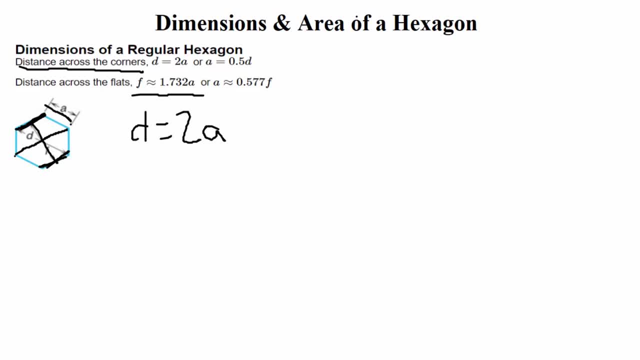 F is approximately equal to 1.732A. So again, just take A, the side of the hexagon, and multiply it by that decimal. So for those it's fairly simple. as long as you know what A is, You can calculate the distance across the corners. 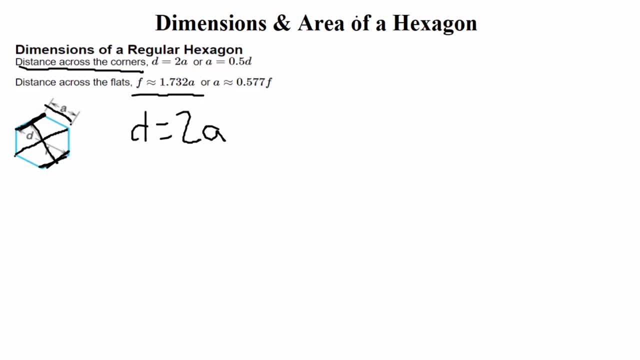 the distance across the flats. So let's go ahead and try an example. Okay, so over here at the bottom of the screen, I have an example of a regular hexagon, and we're given that the side is 10 centimeters. 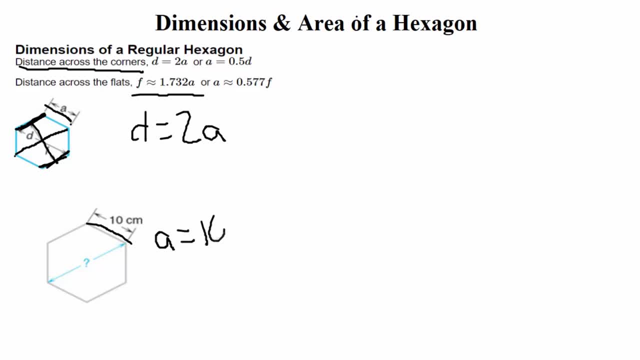 So that's what A is. A is equal to 10 centimeters And noticing what we're looking for. so we see this question mark here, this line that goes across. So first off, we need to pay attention. Is it asking us for the distance across the flats? 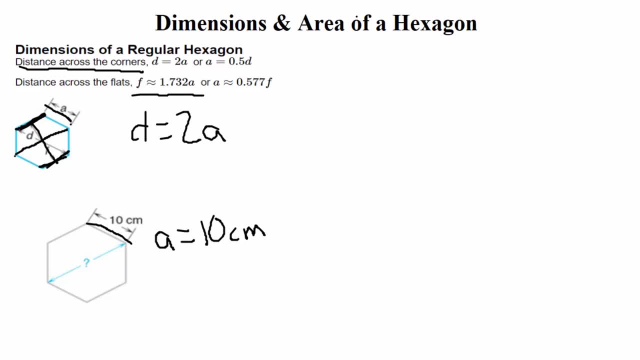 or is it asking us for the distance across the corners? So, taking a look at this one, this one goes from corner to corner. right, It's not the flat side, It's the corner to the corner. So therefore we need the formula for distance across the corners. 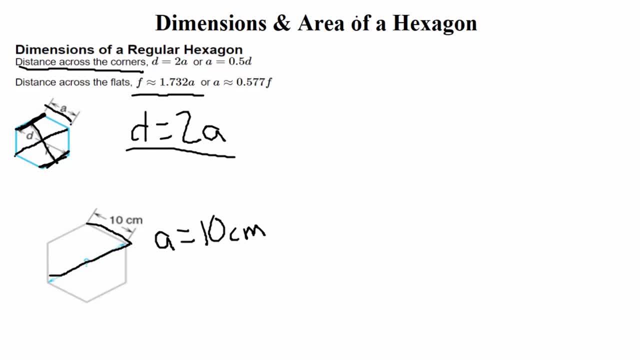 And that's the one that says D is equal to 2A. All right, so we can take D. That's what we're solving for. We're going to take 2 and multiply it by A. D is 10 in our example. 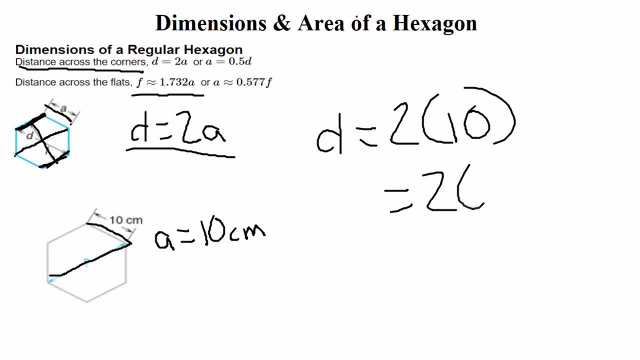 So this is just a matter of calculating 2 times 10.. So that means the distance across the corners would be 20 centimeters. Now, even though this particular question isn't asking us, let's go ahead and calculate the distance across the flats. 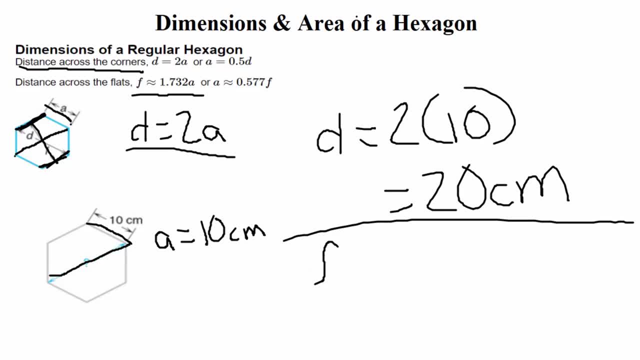 All right, we can do that here. So if we're finding the distance across the flats, that formula is: F is approximately equal 1.732A. So for that one here all we would have to do is plug in A there. 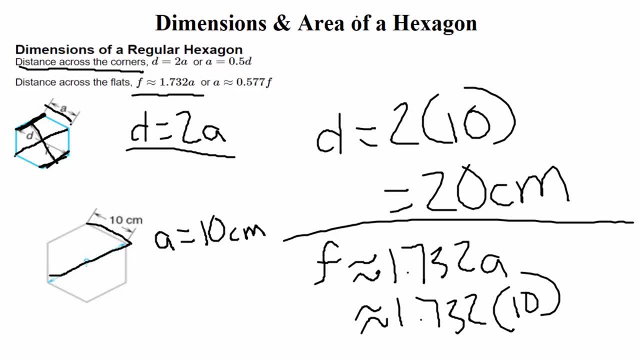 Which would be a 10, right. So 1.732 times 10 is going to give us 17.32 centimeters. So now we know the distance across the corners, We know the distance across the flats. So just depending on what you're being asked for for a particular problem, 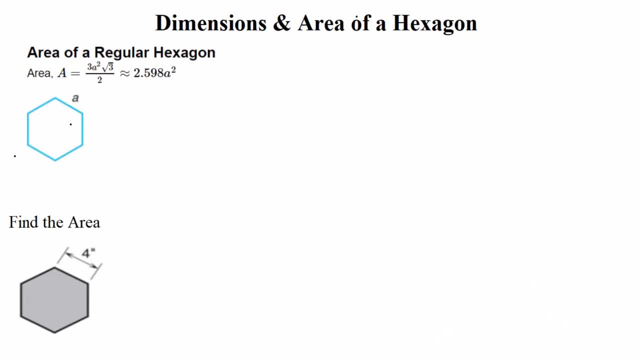 Okay, so here I have another hexagon down at the bottom of the screen, But for this one here we're going to focus on how to find the area of it. So at the top of the screen I have the formula for finding. 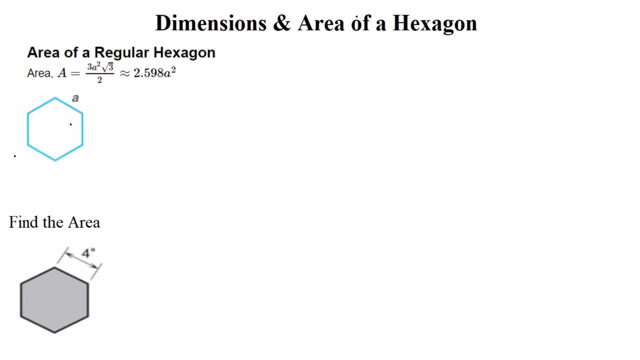 the area of a regular hexagon. All right, so we're given that the area is equal to 3A squared times the square root of 3 divided by 2.. But they've kind of broken down some of that calculation for us. 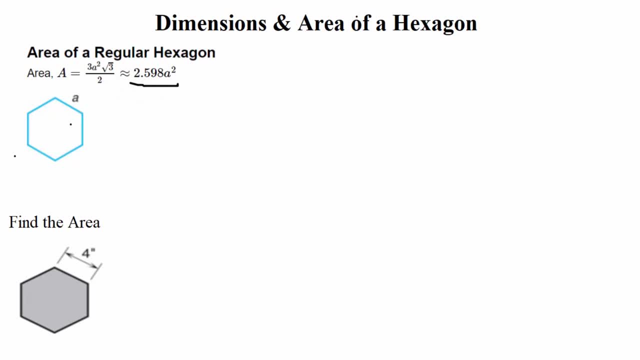 which is good and makes the formula a lot easier to calculate. So the formula that we actually need is the 2.598A squared. So that's the formula that we're going to want to use for our purposes here. It's a simplified version of the formula that's going to make. 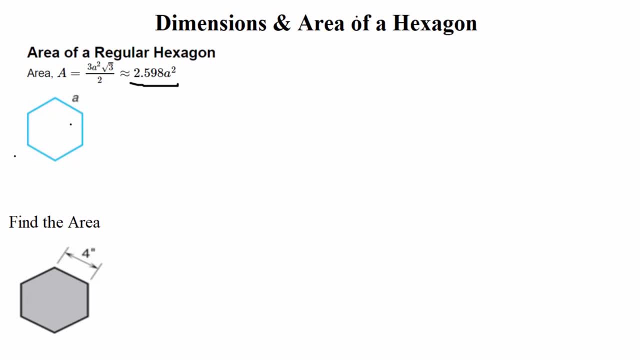 our calculations just slightly easier here. Okay, so taking a look at the example that we have at the bottom here, the only thing that we're given about this, other than it's a hexagon here, is that the side is 4..